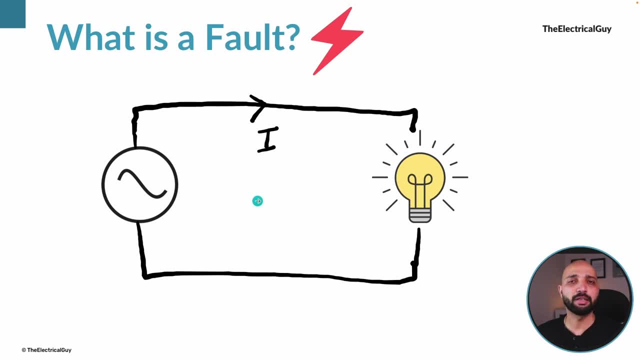 the intended path for the current. Now, let's say, one of the life part of this circuit is now touching the ground right. So here you can see. what has happened is the current is diverging from its intended path. Now it is flowing through this low impedance path which is offered by this. 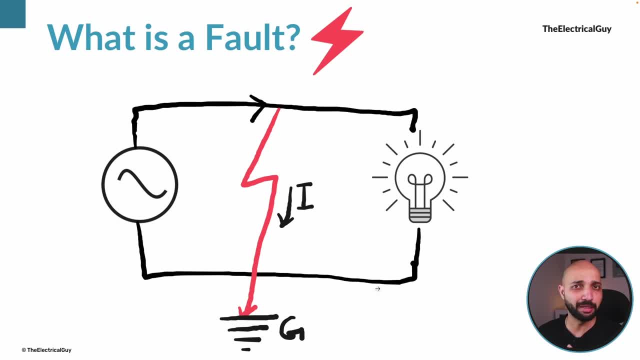 red line. Now, if you want to know what is impedance, which is the term most commonly used in AC circuits, I have a detailed video on that. You can check it out. Link is provided down in the description. Now, since there has been a fault- there has been, you know- the life part is touching the ground and, as 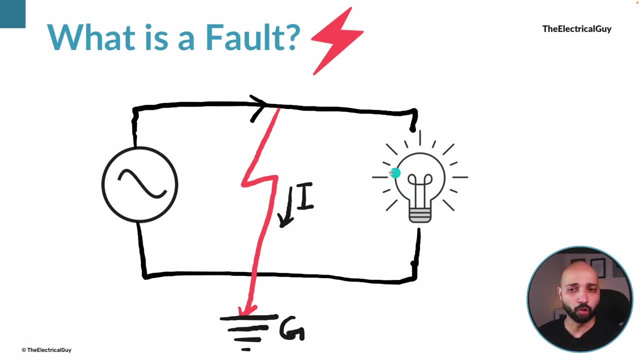 a result, the light bulb is not glowing and current is flowing through this red path right here, and this type of situation, wherein the current is diverted from its intended path, is what we call as fault right, It is very easy to understand. So, a situation in which current in a closed circuit is 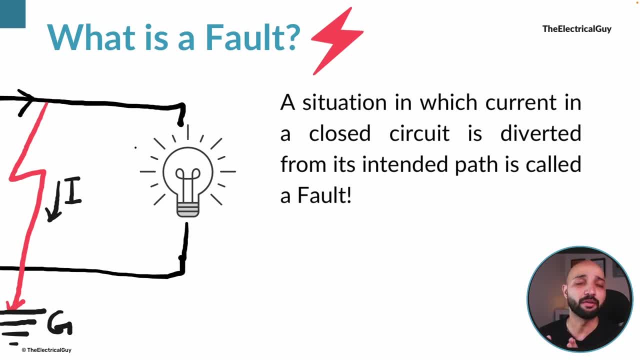 diverted from its intended path is called a fault. Now, since the fault impedance is very, very low, the amount of current in case of a fault becomes very high and we call that situation as abnormal situation or abnormal condition. It can reach to many kilo ampere, So that is what we call as fault. 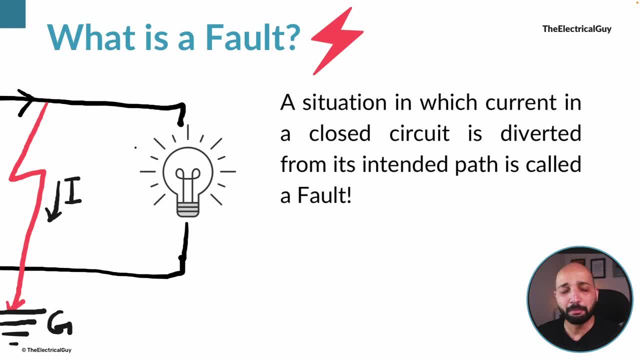 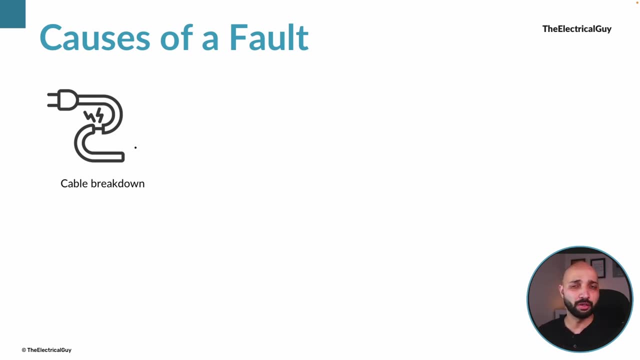 in very simple language Now. there can be multiple reason why current is diverted from its intended path. There are multiple reasons for that. Let us have a look at some of them. So one: there can be a cable breakdown which is causing the current to go to a different direction than its intended. 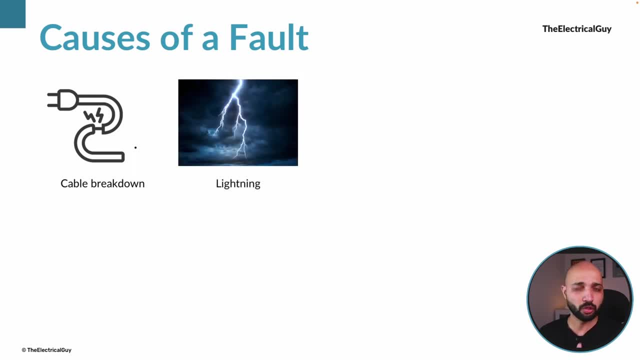 path, or there can be a lightning stroke which is causing the fault, or maybe the flood situation or high-speed wind that will cause transmission line to you know, two transmission lines connecting each other. Then there can be trees falling on the line. This is generally seen in the distribution. 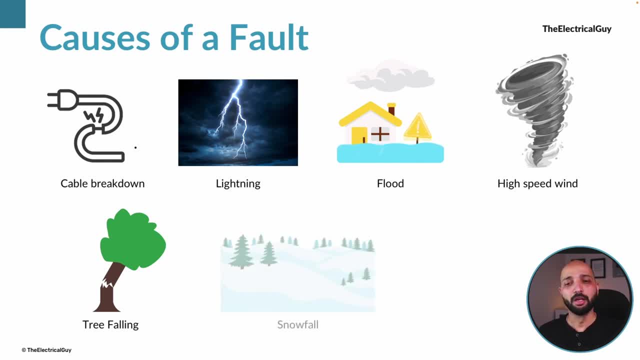 network and also to some extent in the transmission network or so on and so forth. So there can be a snowfall that happens on the equipment and also on the transmission and distribution lines, or there can be situations like earthquake. Now, if you see, majority of the situation right here is natural in. 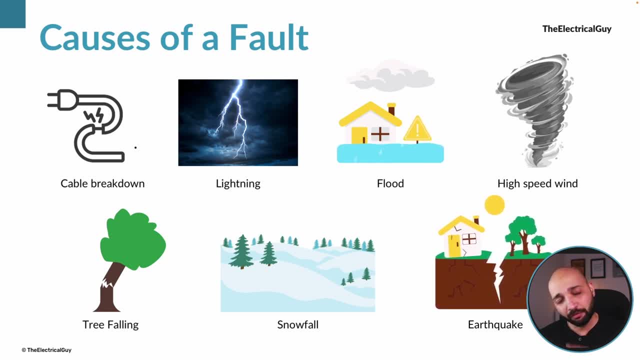 nature. but there can be a situation in which the equipment itself failed or equipment malfunctioned and that can cause current to divert from its intended path, and which is nothing but default. or it could be a man-made situation also, for example if somebody is carrying out maintenance and during that period the connection of the equipment is done wrong. So that can also. 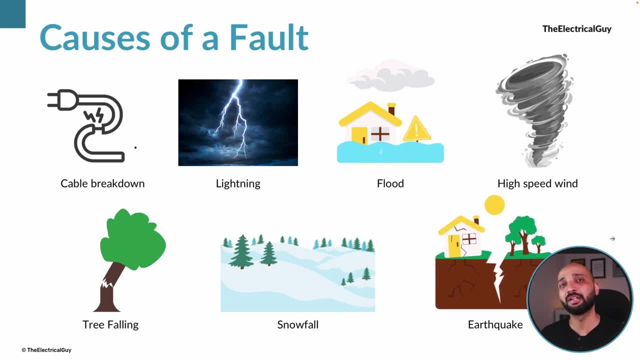 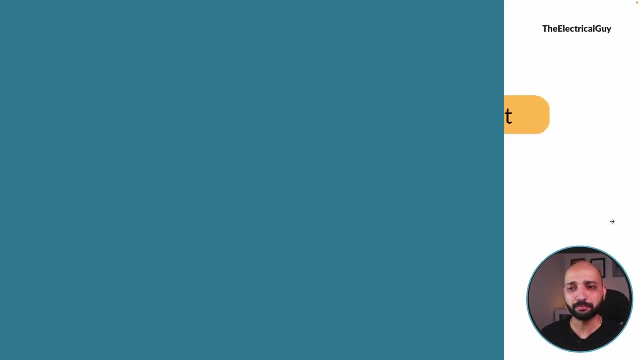 cause fault and, as a result, in that case, current can go up to a very high level, right? So these are some of the reasons why a fault can occur. Now let us talk about the different types of fault that we have seen in the power system. So, on top level, if you see the, there are two. 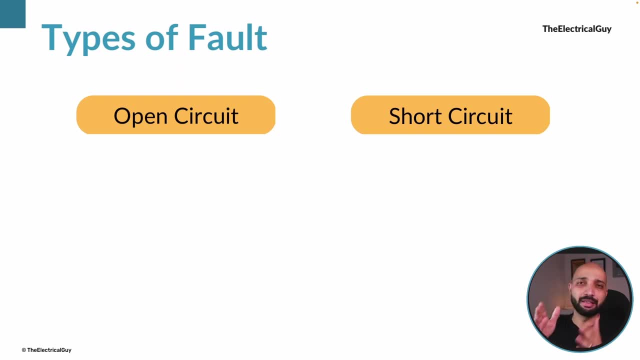 main types of fault. One is the open circuit and then there is a short circuit. First let us talk about the open circuit and then we will also talk about short circuit in few minutes. So, talking about open circuit, let us say we have three phases- R, Y and B- and one of the phase is broken down in between. 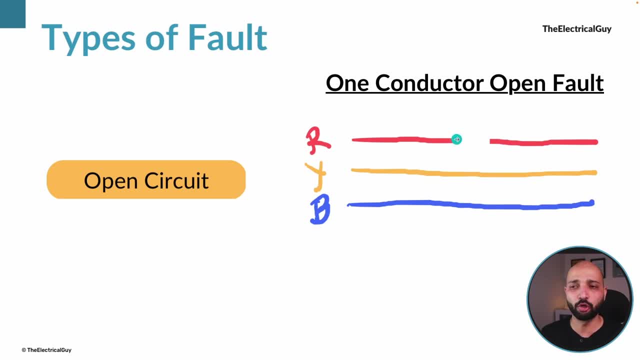 and, as a result, the current will not flow beyond this point. it is getting stopped, it is opened. basically, So this is nothing but a short circuit. and then there is a short circuit, and then there is a open circuit fault, and if you are interested to know in detail about open circuit, then I have a. 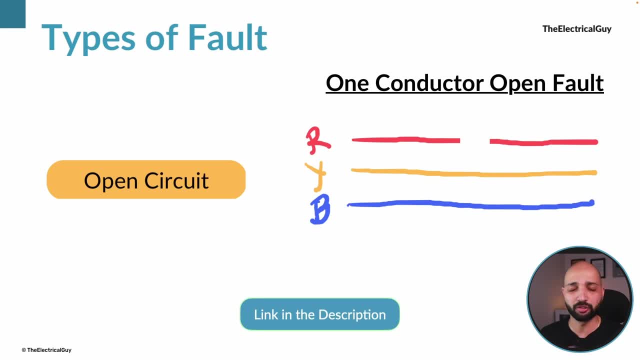 detailed video on that. again. I will provide link for it down in the description. Now, here you can see, the R phase is broken down. so out of three, one phase is down. So this fault is called as one conductor open fault. Now in open circuit what will happen is, since this conductor is broken, 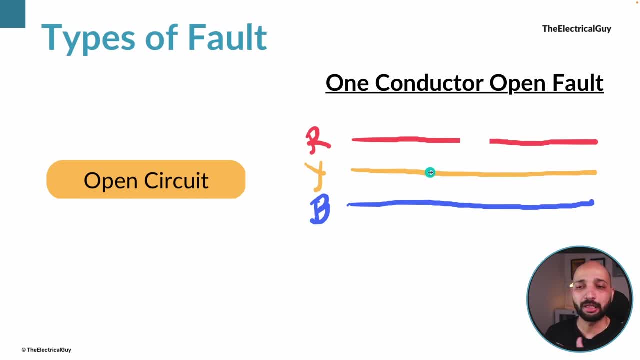 the load of this conductor will be then on Y and B phase, So definitely these two phases will have to carry additional load. as a result, the temperature of the conductor will increase and that will create further issues in the power system. So definitely this fault also needs to be. 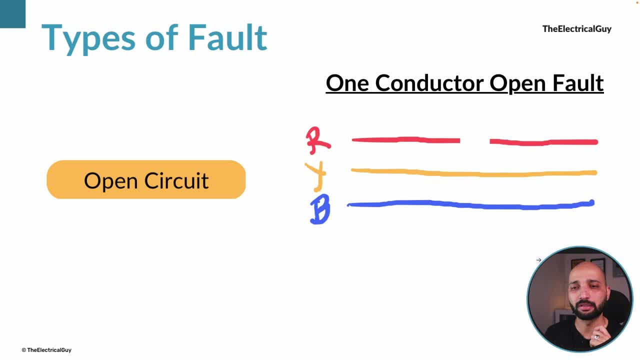 avoided or there can be a situation, let's say, in that case Y phase is also broken down. Now, here you can see, out of three, two phases are broken down and such type of fault is called as two conductor open fault. Two conductors are open, or maybe 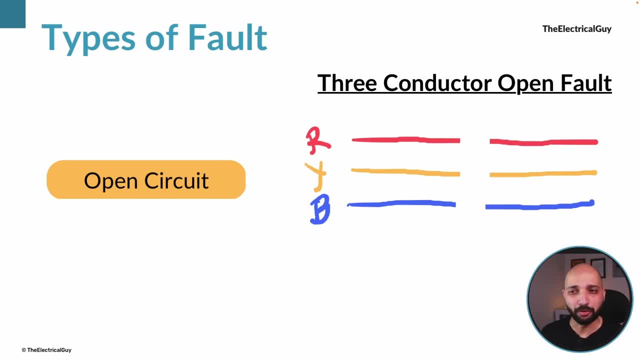 there can be a situation where all three phases are gone down and that fault we call it as three conductor open fault. Now the severity of this fault is not high as the short circuit fault. Definitely short circuit faults are more severe when we compare it with the open circuit fault. 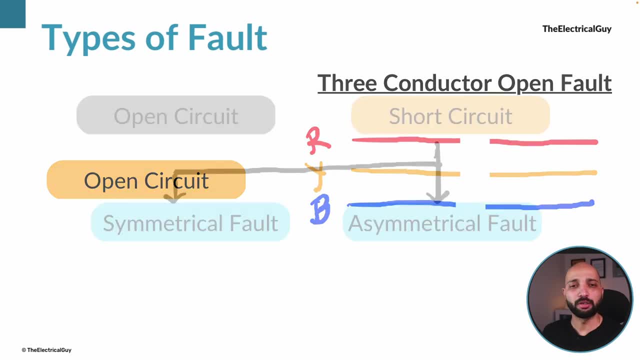 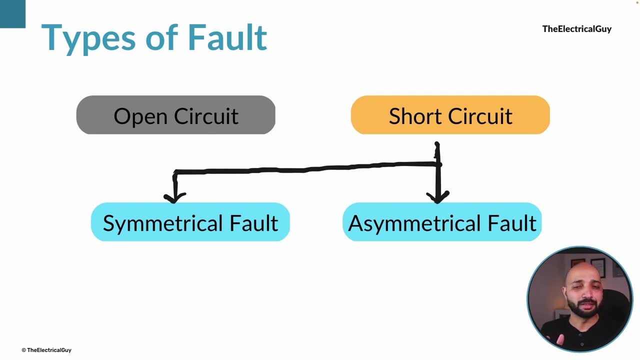 Right, So that is the open circuit fault. Now let us talk about the short circuit. Now, short circuit faults are basically divided into two types again. One is symmetrical fault and another one is asymmetrical fault. Let us first try to understand the concept of what is symmetrical and what is asymmetrical. So symmetrical is very easy. 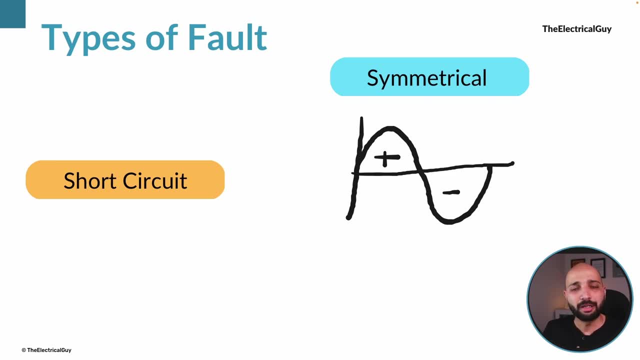 to understand basically. So what do we mean by symmetrical? Symmetrical means both the cycles, that is, positive cycle as well as the negative cycle, are equal. So the peak point of both the cycles are equal. In that case, we call it as a symmetrical fault. Now let's 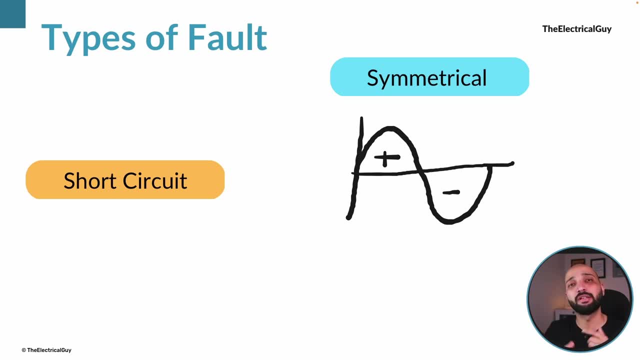 look at a symmetry, a symmetrical situation, and that is generally seen in the balanced load. Now you can see here on the image also, the positive half cycle and the negative half cycle are exactly equal and opposite to each other And such situation is called as symmetrical. 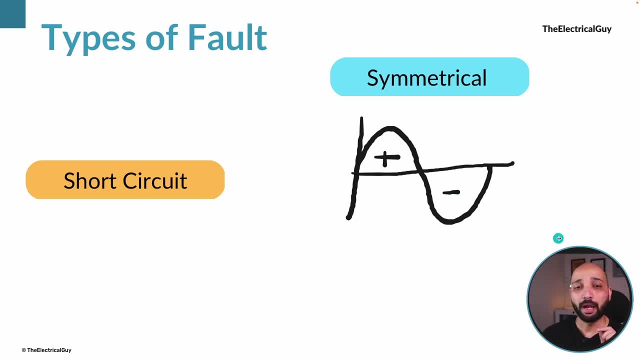 This happens in the balanced load And opposite to that, in an asymmetrical situation, one of the cycles will be bigger than the other. or in simple language, we can say: the positive half cycle and negative half cycle are not equal to each other And that is not in symmetry and that is what we call as asymmetrical And this is generally seen. 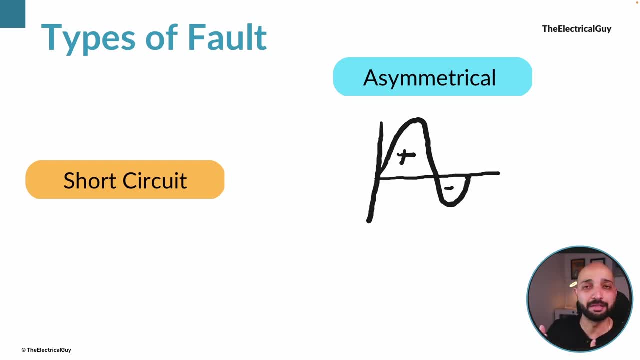 where the system is not balanced. Again, if you are interested in knowing what is balanced and unbalanced system, then I have again a very easy to understanding video on that. link is provided down in the description. So understood the basics of symmetrical, Symmetrical and asymmetrical- very easy to understand And, based on this, the faults. 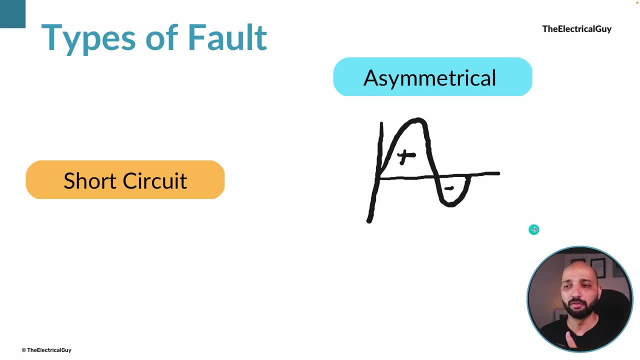 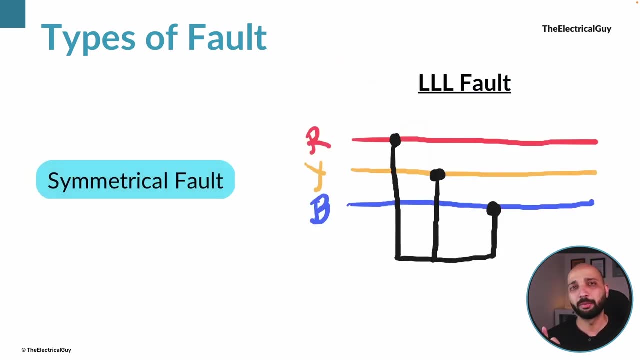 are basically divided, based on this situation, which we will see in few minutes now. Now, first, talking about the symmetrical fault. The first fault in the symmetrical is line triple line fault, So LLL, triple line fault. Now, in this fault, what is happening is all. 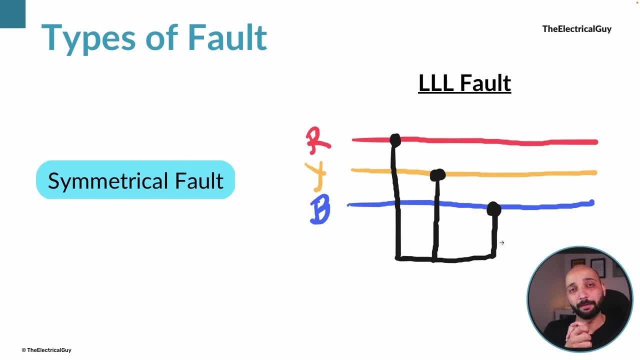 the three phases are somehow getting connected to each other And the fault current that is flowing through the system is equal in every phase, And that's why this fault is called as symmetrical fault. So earlier- I mean before fault- the system was already stable, already balanced, and before fault also. 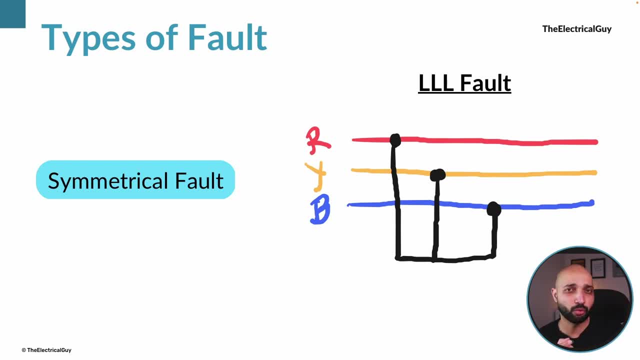 the system is still balanced because all the three phases are connected together and, as a result, equal amount of fault current is flowing through all the three phases, And that's why it is in perfect symmetry And hence it is called as symmetrical fault Clear. 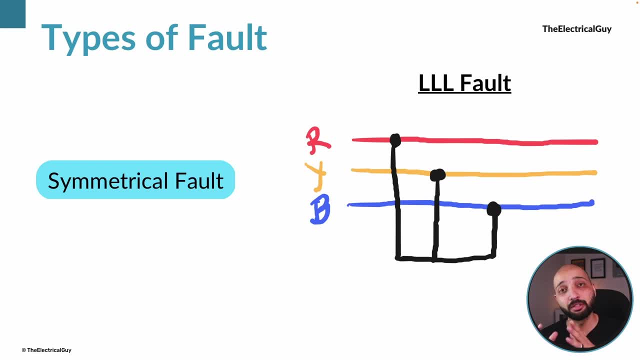 So you may ask: if in symmetrical fault the system is still balanced, does that mean this is a good fault? Well, no, No fault is good actually. Or rather I would say, this fault, triple line fault, is the most severe fault that power system can see, or power system. 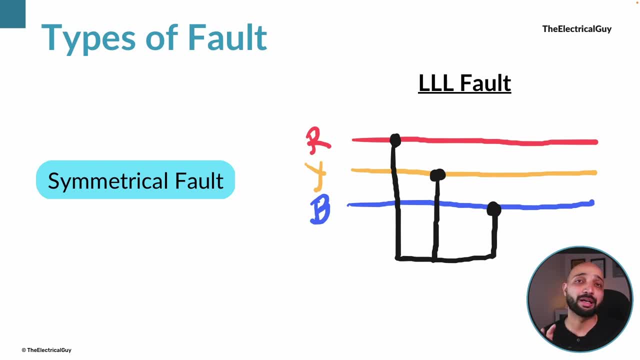 can witness And based on this fault the rating of circuit breaker is decided in majority of the cases. But occurrence of this fault in power system is very, very rare. Now first, very rare if you see, only one to two percent of fault are symmetrical in nature out of total. 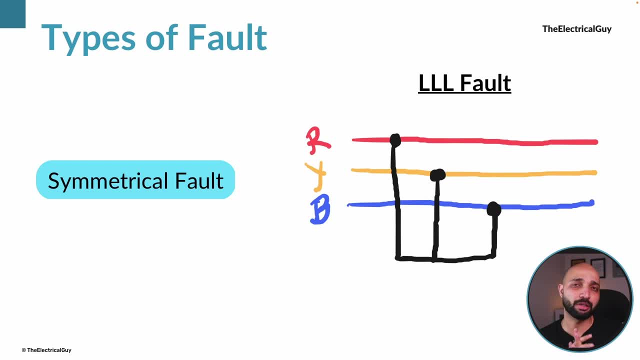 hundred percent faults. only one or two percent fault are in symmetrical nature. but if this happens then it is a very, you know, severe fault. the short circuit current in case of symmetrical faults are very, very high. right, this is the first type of fault which is symmetrical, that is triple. 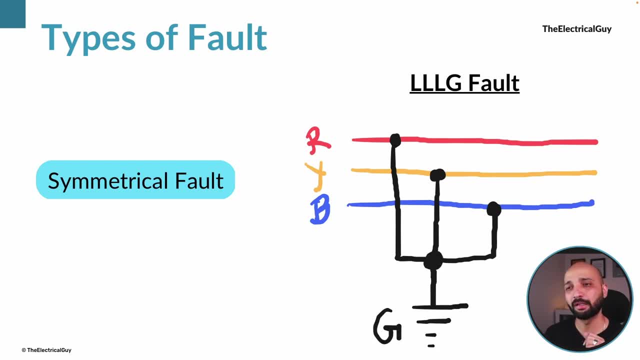 line fault. now. next, one more fault is there and that is called as triple line to ground fault. now in this fault all the three phases are connected, but along with that the ground is also connected, and this is again also one of the severe fault. but occurrence of the fault is very 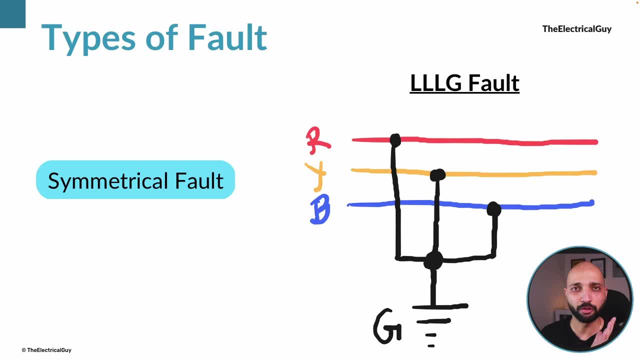 very rare when we compare it with the other faults. so two types of fault in symmetrical triple line fault and triple line plus ground fault, clear that is symmetrical fault. now, moving on, we have a symmetrical fault, so the first one that you can see is line to ground fault. 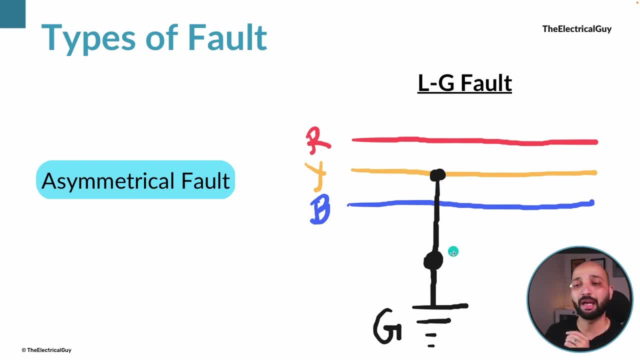 now, in this fault you can see one phase and the ground is connected. so here in our example, y phase and the ground is connected. this is called as single line to ground fault and this is the most common type of fault that you will see in the power system. almost 70 to 80 percent of fault are 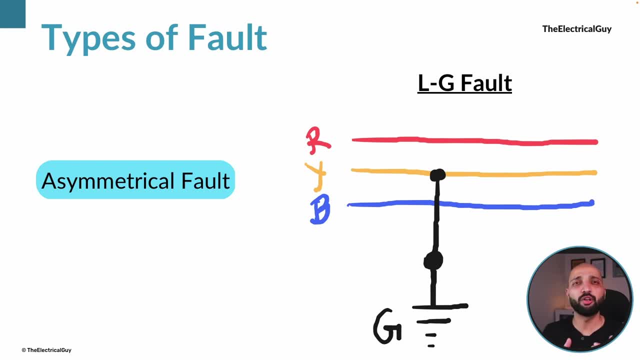 line to ground in nature. this is the worst type of fault in nature. the severity of this fault is not high as the symmetrical fault that we have seen, but this is the most common type of fault that you will see. line to ground fault again. there is one more variation in that and that is a double line fault. now here you can see y phase. 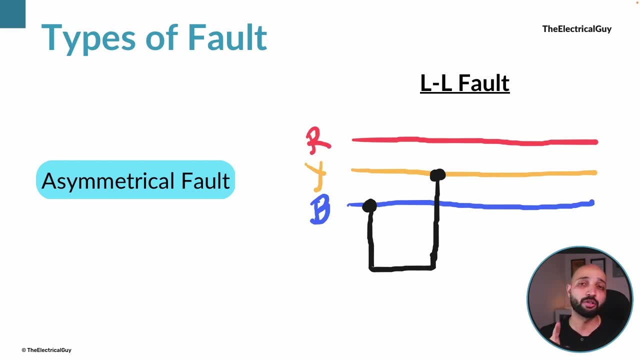 and b phase are connected together. again, it is a symmetrical fault because your r phase is healthy and y and b phases are not in a healthy situation. so definitely current flow is very low in nature. flowing through all the three phases will be different, which will result in the asymmetry. 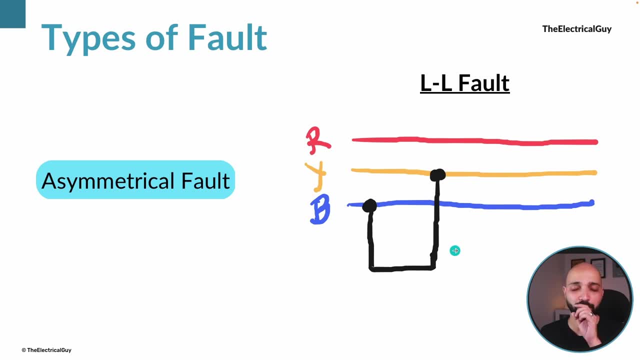 clear. so that is double line to double line fault again. there is one more variation in that, and that is double line to ground fault. now, here y and b phases are connected together, plus the ground is also into the picture. so this is a double line to ground fault clear. and these, all these are: 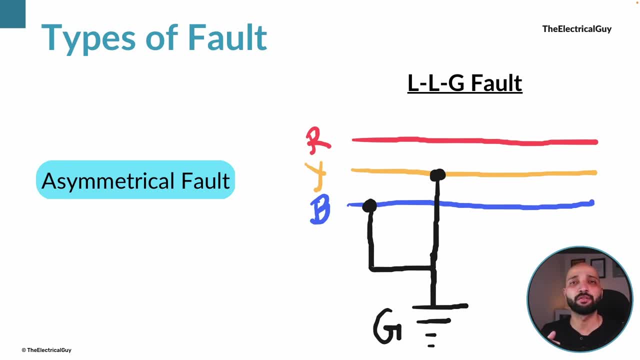 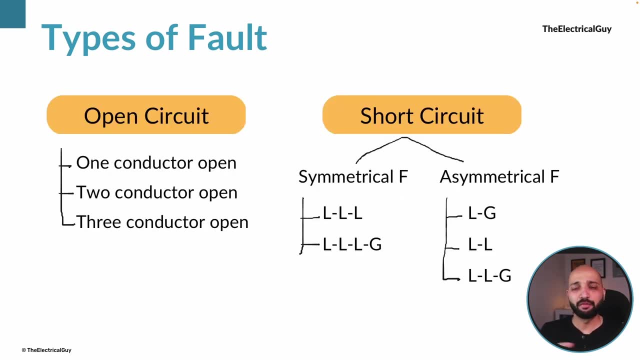 asymmetrical fault. the positive half cycle and negative half cycle in such faults will not be equal and hence causing the asymmetry. now let us quickly revise the different faults that we have seen. so there are two main types of faults in the power system. one is open circuit, another one is 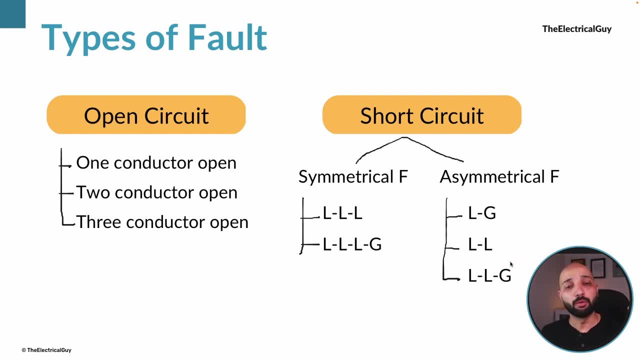 short circuit. in open circuit we have seen one conductor open, two conductor open and three conductor open. the severity of this fault- hours are not high, as the short circuit is the second type of fault are short circuit in nature and again, if you want to know in detail, 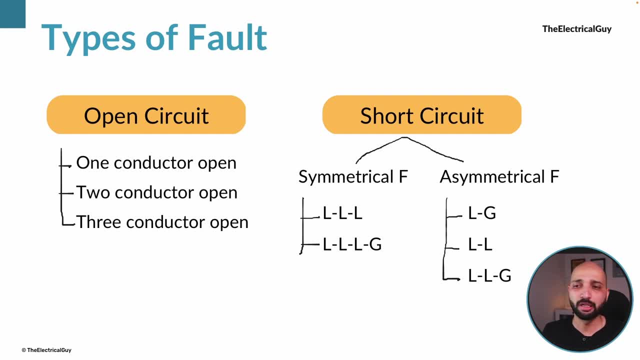 about short circuit. i have a video on that link i'll provide down in the description. so short circuit fault are classified into two different faults, that is, symmetrical fault and asymmetrical fault. in symmetrical fault we have seen two types of fault: triple line fault and triple line plus. 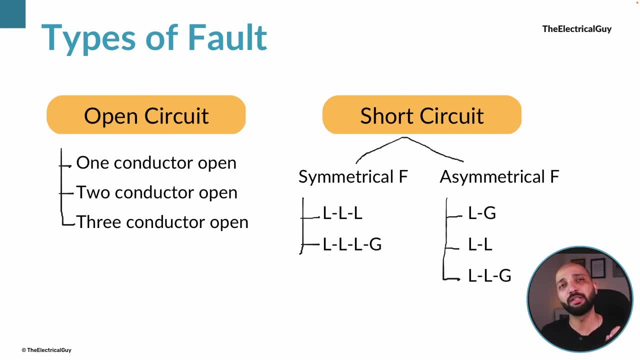 ground fault. the occurrence of symmetrical fault is very rare in power system. only one to two types of fault, and the second type of fault is short circuit in nature. and again, if you want to know in detail about short circuit in nature, and again, if you want to know in detail about: